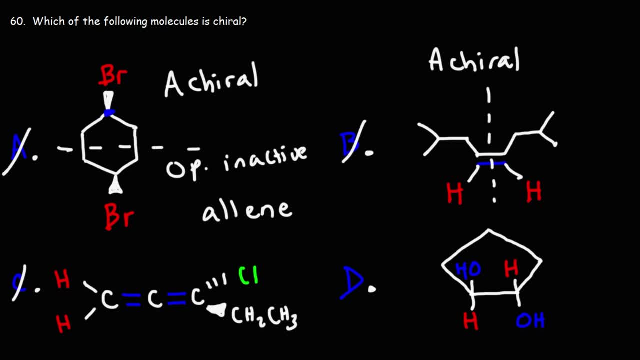 On the right side, we have two different groups. On the left side, we have two of the same groups. If one of the sides have two identical groups, it's going to be achiral. In order for it to be chiral, the right side has to have two different groups and the left side has to have two different groups. 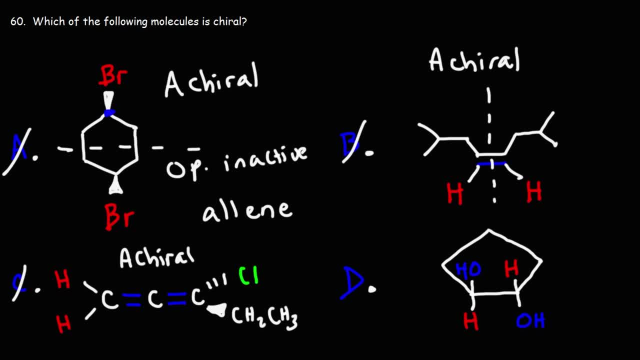 In order for it to be chiral. Now for answer choice D. notice that we don't have a chiral molecule. We only have a plane of symmetry. The left side is not the same as the right side, So this is going to be a 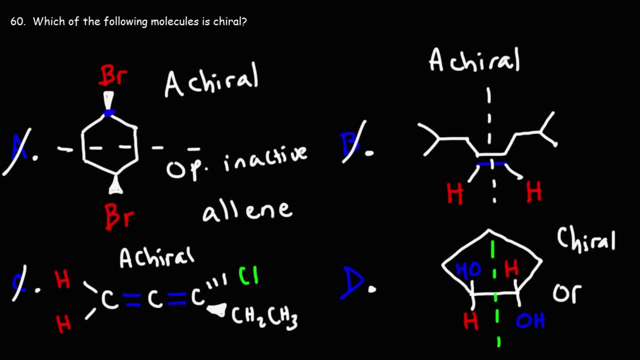 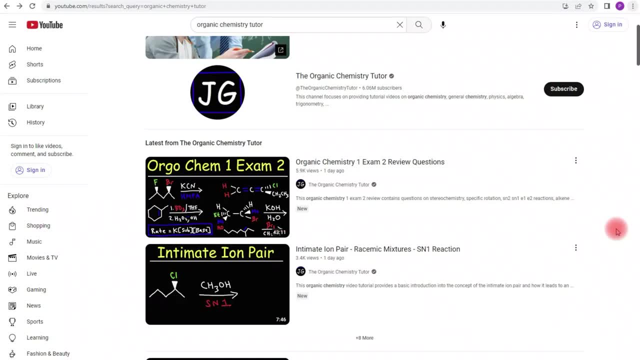 This molecule is chiral, which means it's optically active, So D is the correct answer for this problem. Now, this is for those of you who might be interested in joining my YouTube membership program. If you type in Organic Chemistry Tutor in the YouTube search box and click here, it's going to take you to my channel. 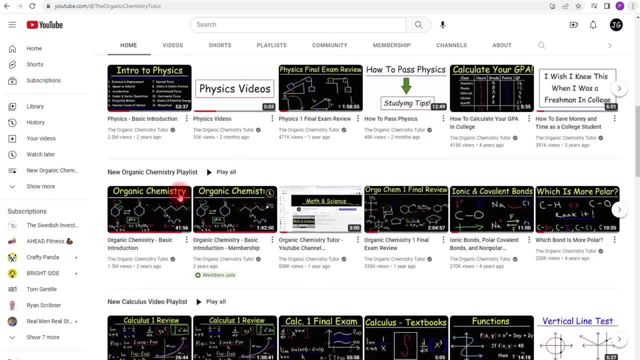 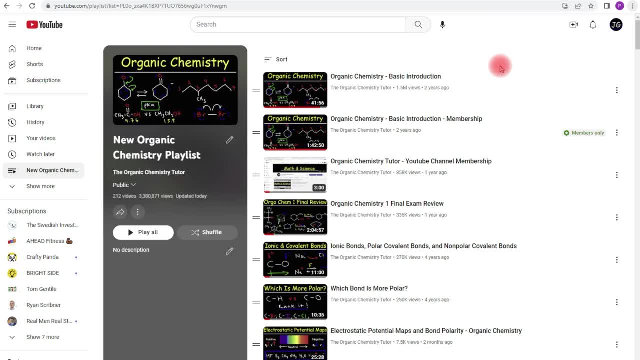 Now, if you scroll down, you could find my Organic Chemistry video playlist And in this playlist you could see all the videos that I have available to those in my membership program. So, for instance, if you look at this video, this is a basic introduction into organic chemistry. 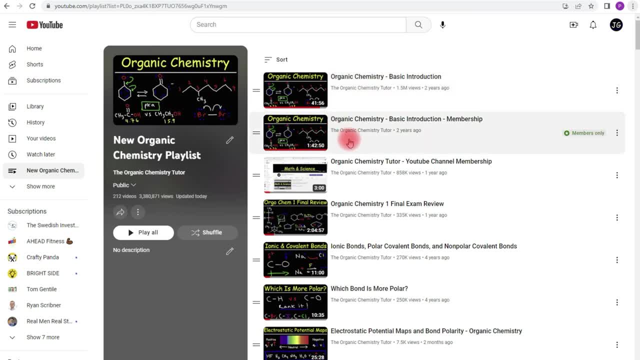 It's about 42 minutes long, but the full version is an hour and 42 minutes long And that's accessible if you decide to join my membership program. But now you not only get that much information, but you also get the full version. 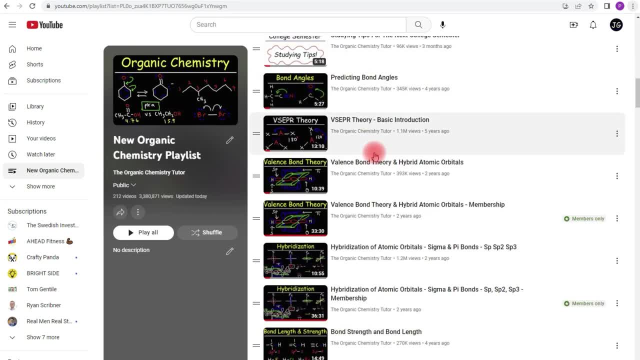 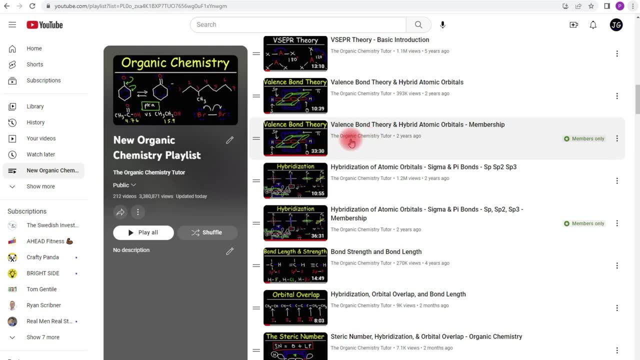 So if you click here, you can see all of my videos, But you also get other videos as well. So, like this video on valence bond theory, you get access to the full version, which is about 33 minutes long, compared to the free version, which is 10 minutes long. 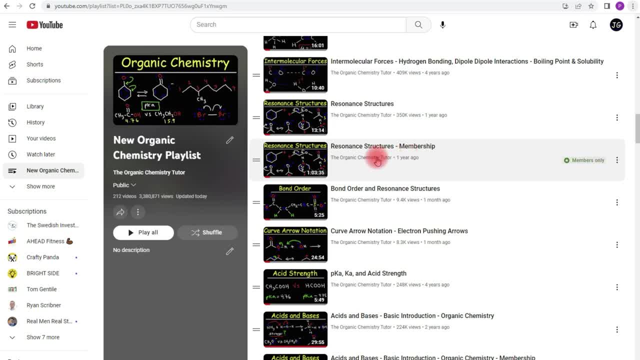 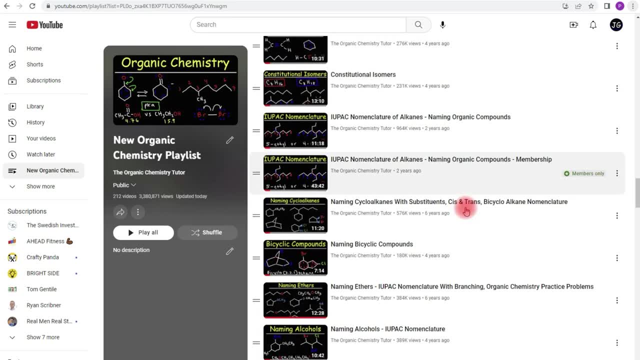 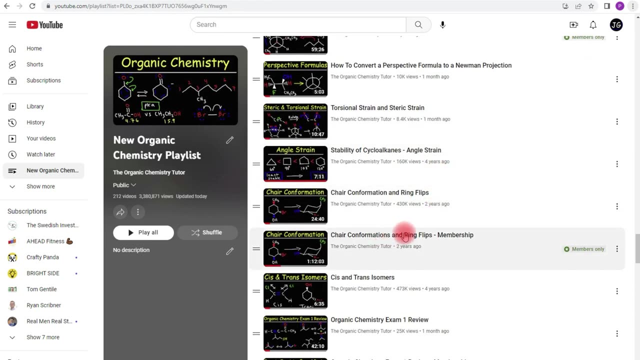 And you could see it here. I have another one: resonance structures, acids and bases, pKa values for acids, IUPAC nomenclature, Newman projections chair. conformations with rings. Now this video is my organic chemistry exam. one review: 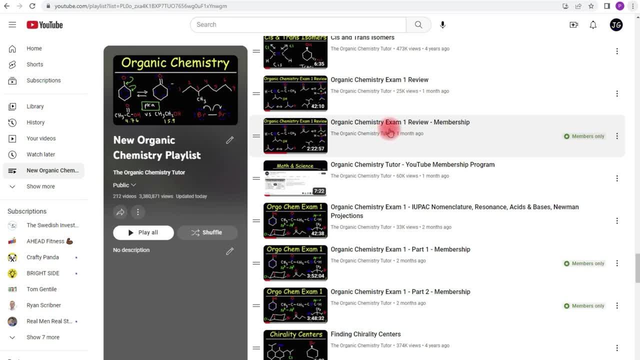 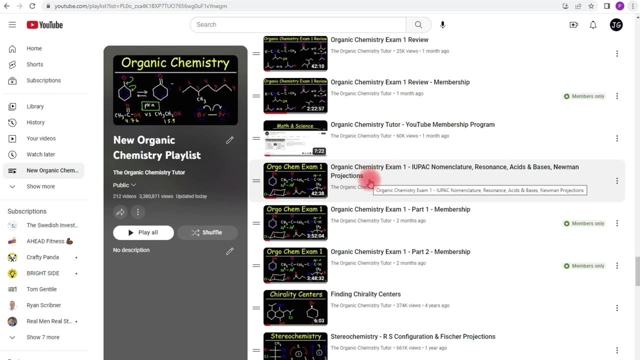 It's a quick review of the things that you'll typically be tested on in the first semester exam of organic chemistry. The free version is about 42 minutes long. The full version is two hours long. Now over here. this is an actual practice exam with multiple choice problems and free response questions. 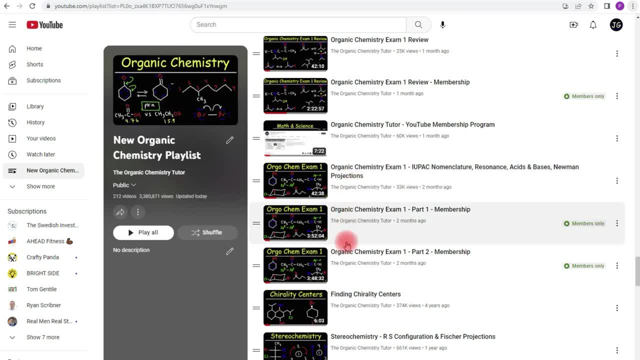 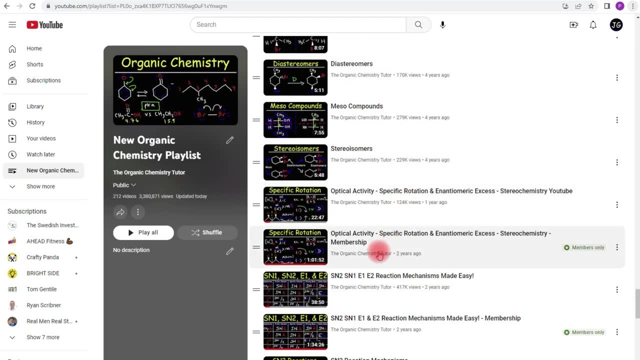 As you can see, the free version is only 42 minutes long. The full version combined is between seven to eight hours long. Now I have other videos on stereochemistry: specific rotation: SN2, SN1, E1, E2 reactions. 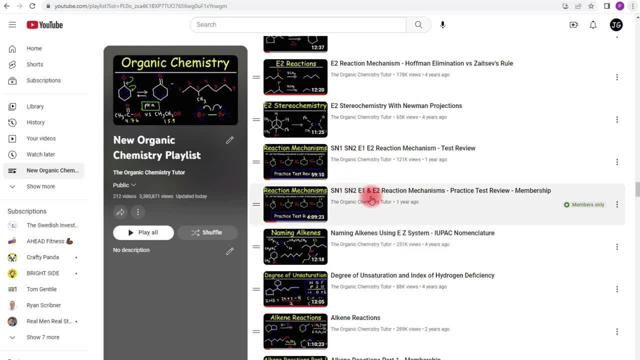 I have a practice test on that, because that's a topic that a lot of students struggle with. So the full practice test is about four hours long. Again, if you join the membership program, you'll get that. If you join the membership program, you'll get access to that video. 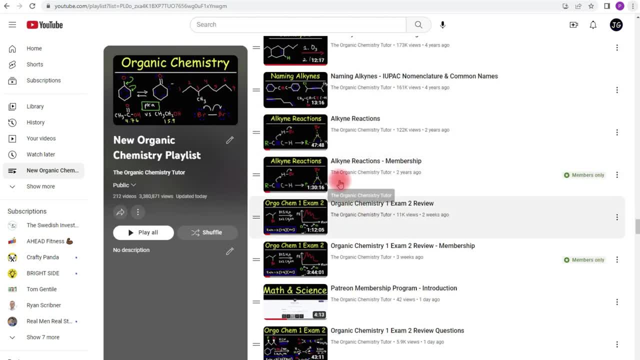 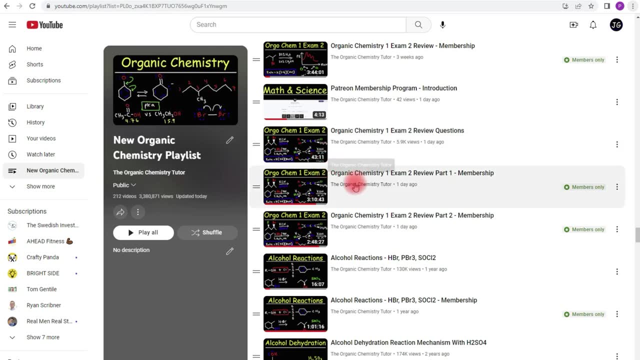 I have videos on alkene reactions. alkyne reactions and this is my organic chemistry. one exam, two review Over here. this is the practice test, with about 85 questions. As you can see, the full version is six hours long. 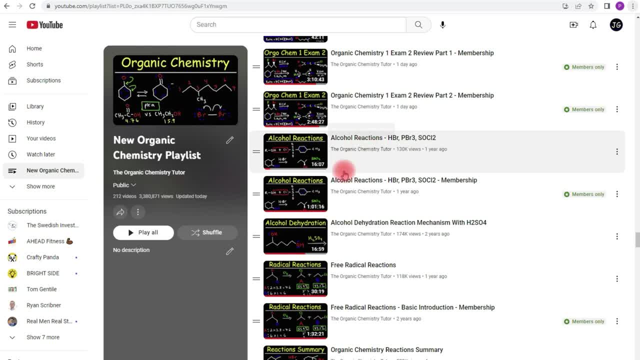 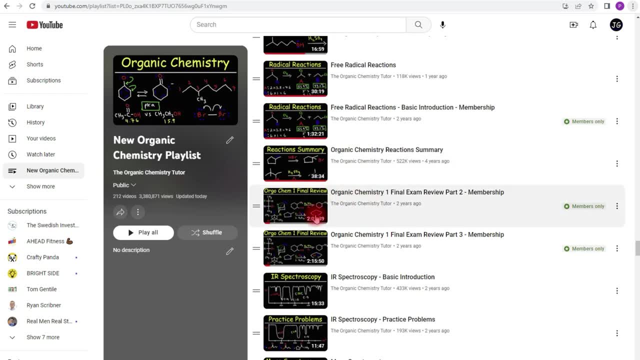 The free version is about 43 minutes long. In my membership program you'll get access to alcohol reactions, free radical reactions and, of course, my organic chemistry. one final exam review video. The full version is about six hours long, but the first two hours are free. 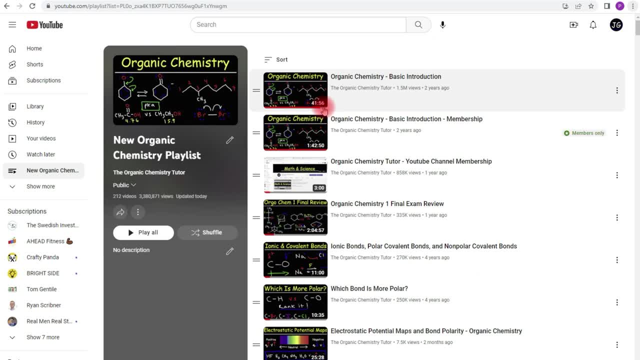 This is the last four hours. To find the first two hours that are free here, it is right here at the top of the list, So feel free to take a look at that if you want to know what you're getting if you decide to join my YouTube membership program. 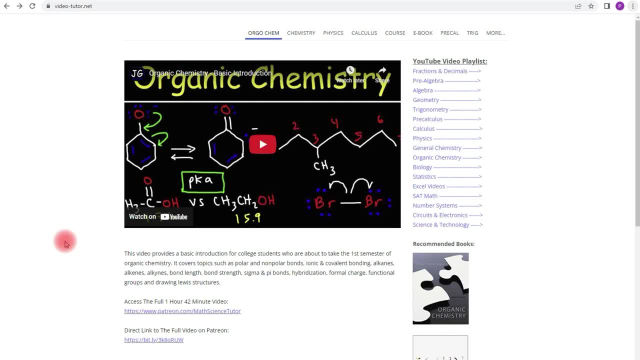 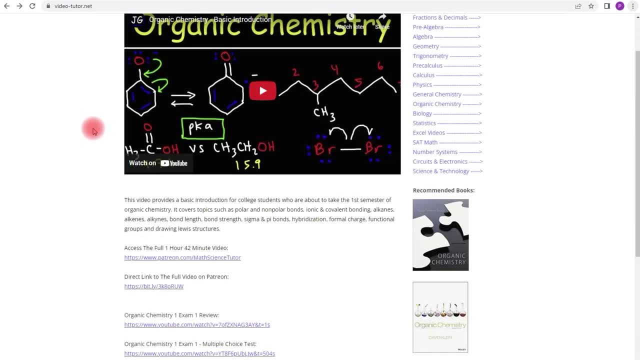 Now, this is for those of you who want to get access to all of my video playlists. You can get access to all of my video playlists and exam review videos all in one spot. So if you go to video-trudanet and if you go here, click more video playlists. 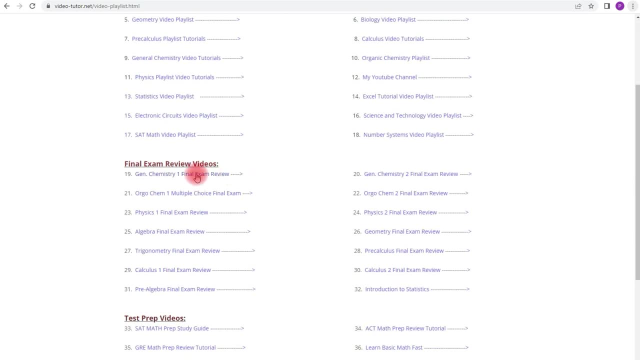 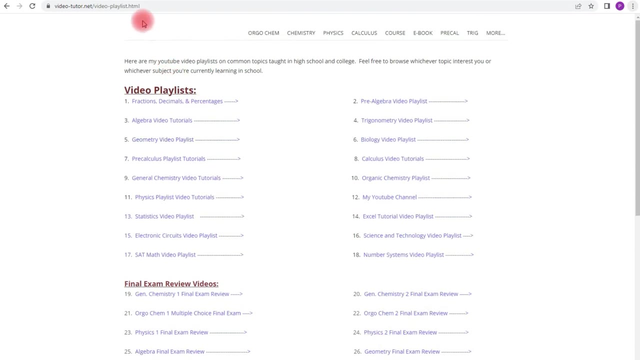 you can get access to all the different video playlists that I have on my YouTube channel, and also the final exam review videos as well, So feel free to take a look at that when you get a chance.